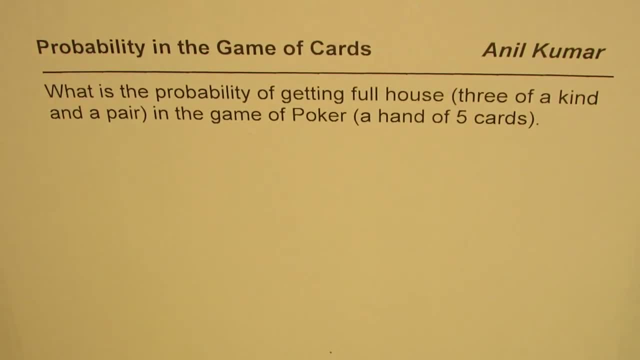 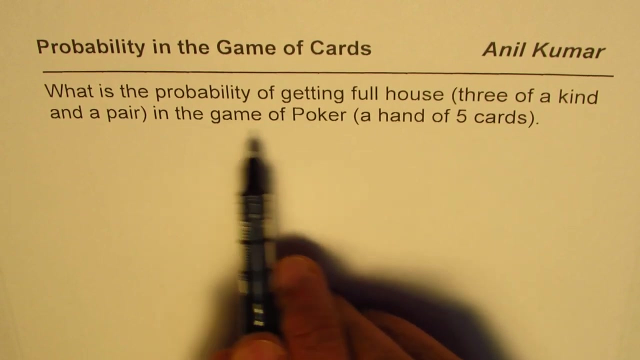 I am Anil Kumar. We are trying to understand probability in the game of cards. Here is an example: What is the probability of getting full house? Full house means three of a kind and a pair in the game of poker. In the game of poker we give five cards, So in a hand of five cards. So that is how you could really understand the question. So what we are doing here is we are trying to find probability in the game of cards. 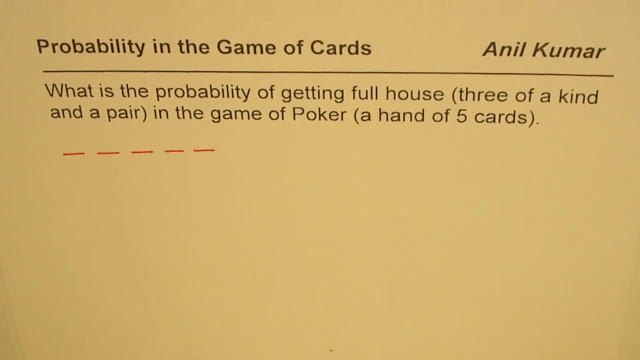 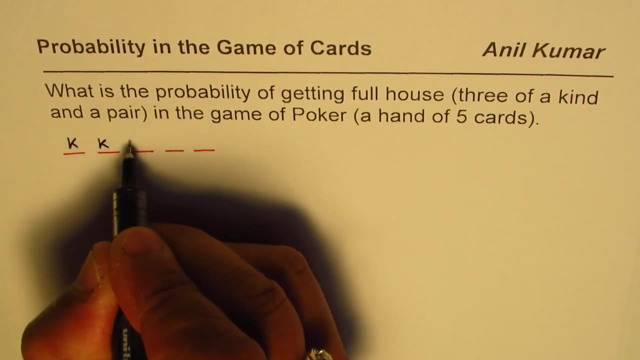 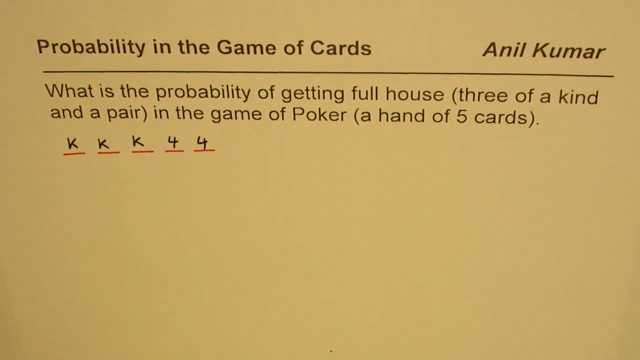 So let's say that out of five cards, we have a full house. Full house will mean three of a kind. Three of a kind means, let's say, we have three kings, Right, Three kings And a pair- So something else It could be like this- And a pair. So what is the probability of getting this kind of a card? So that is the question for you. Let us see how to solve this. 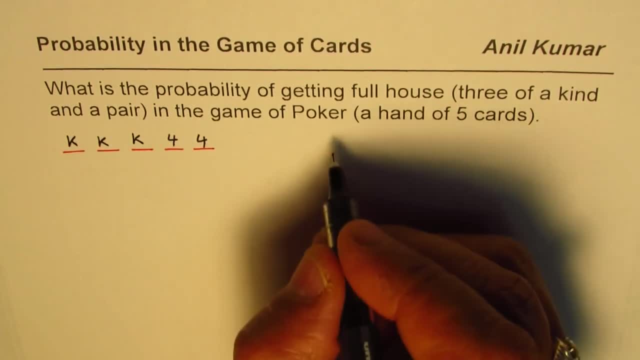 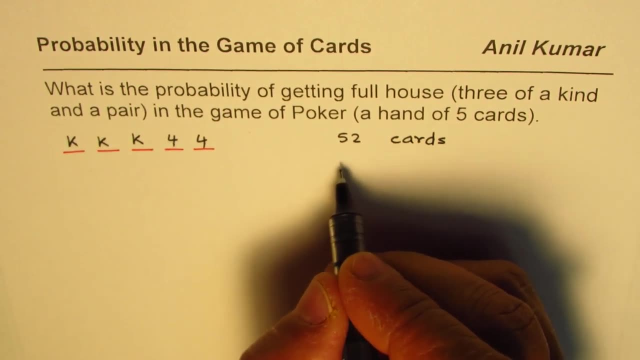 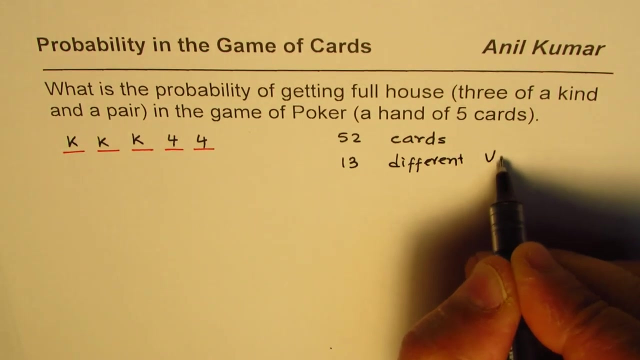 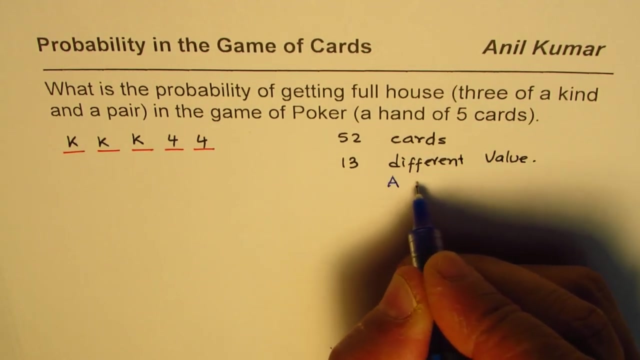 Now we know in the game of cards we have 52 cards Right, So their value is 13 or different values. 13 different values, Values we mean ace king queen, like this: Ace king queen jack. These are the face cards. 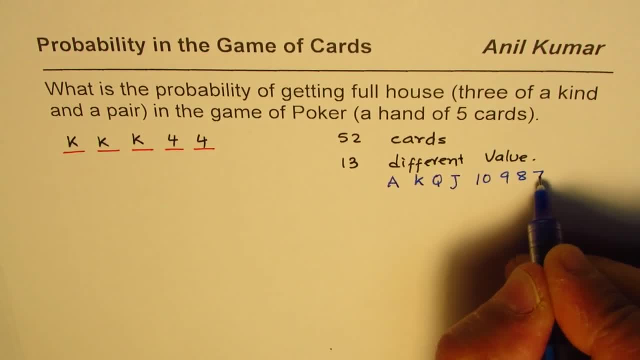 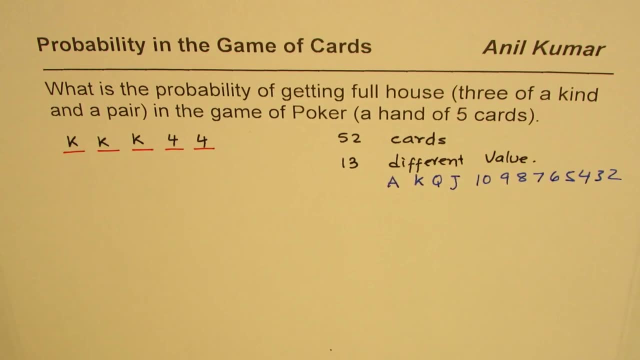 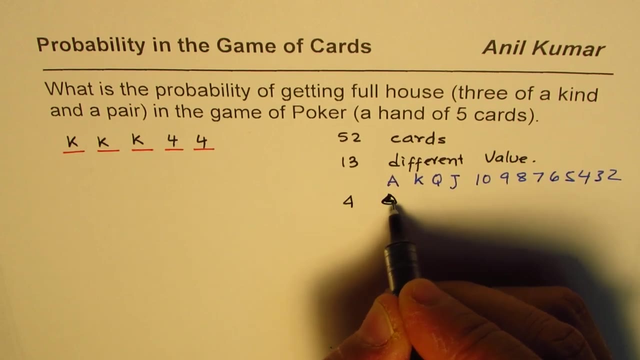 And then we have numbers 10, 9, 8, 7, 6, 5, 4, 3, 2.. So these are the 13 cards with different values, And we also have four suits. Four suits are spades clubs. These are the two black suits. 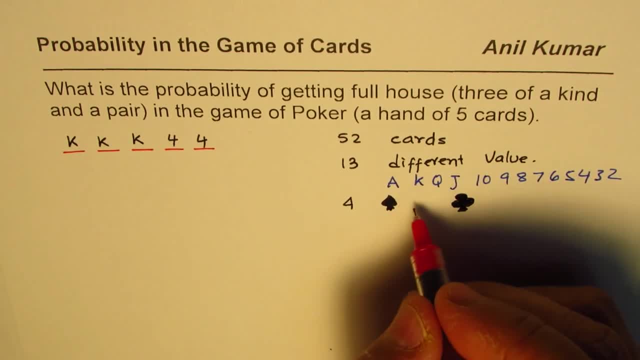 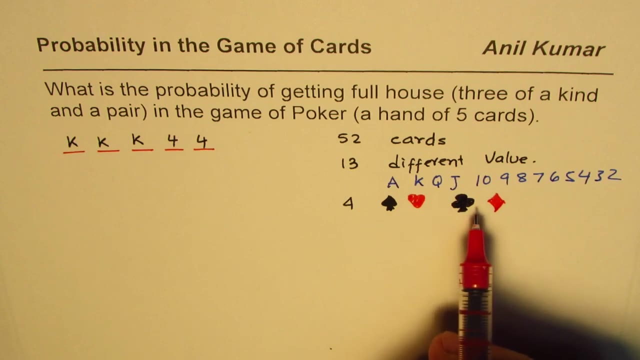 And then we have two red. These are the two black suits are hearts and diamonds. So every card could be of 4 types. so that means 13 times 4 is 52, right? So that is how we have the distribution of cards. Now, to solve this question, we 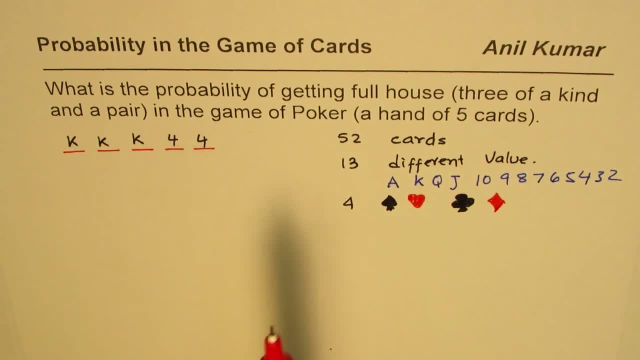 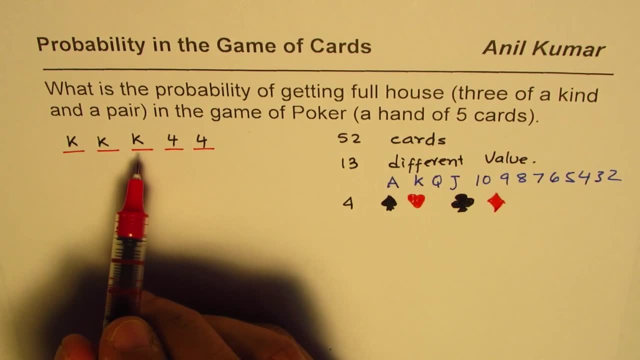 are looking for 3 of one kind and 2 of another kind. So let us see how to do this kind of a question. So the first step here is: let's find the value of card for 3 of one kind. 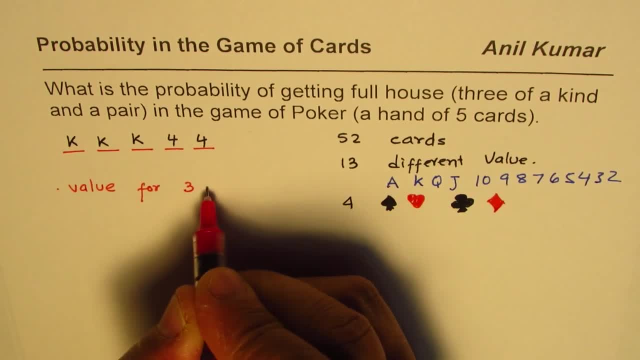 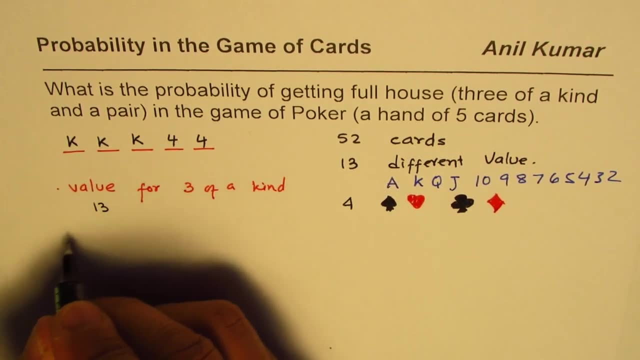 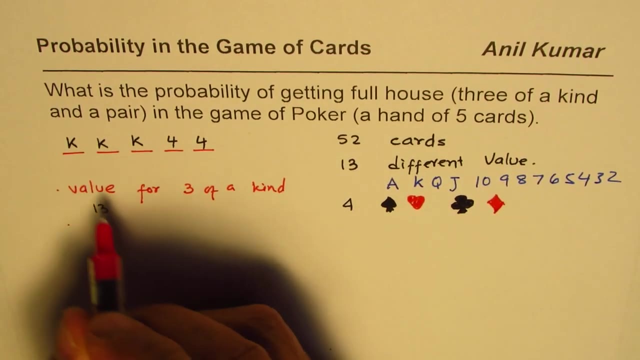 So value for 3 of a kind right. So we could select this value from 13, right? So that is, we have 13 options And how many do we choose? We choose 3 out of those right. So if we select one of these, any one of these, let's. 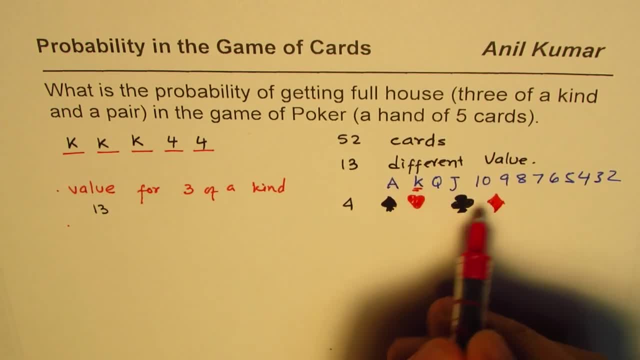 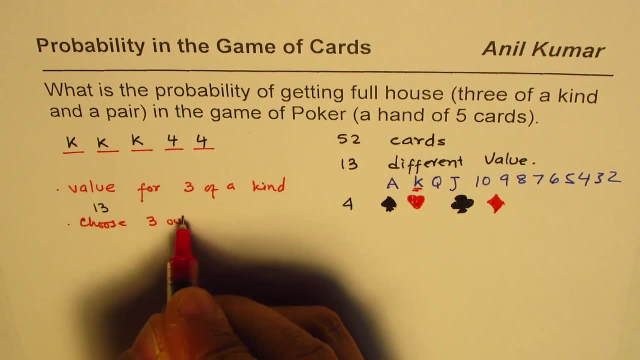 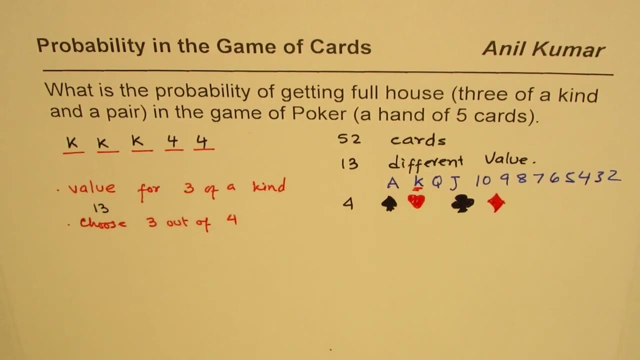 say: we selected king, then we have choice to make from 4 kings, right? So we have to choose 3 out of 4, right of that value. In this case, what we did was: we have selected king here, So we are selecting king. 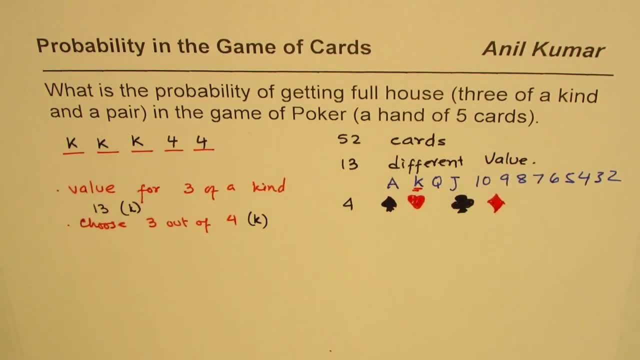 3 out of 4 kings. So that gives us the choice. as from 4, you have to choose 3, right? So that is the first one. Now we have to select the value for the next one. We have already. 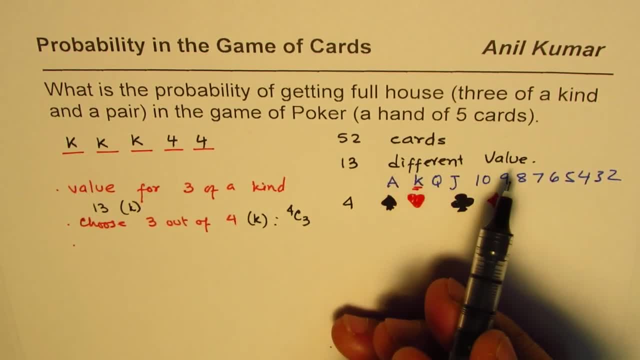 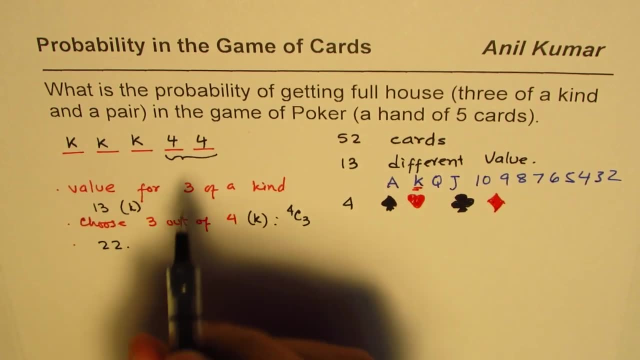 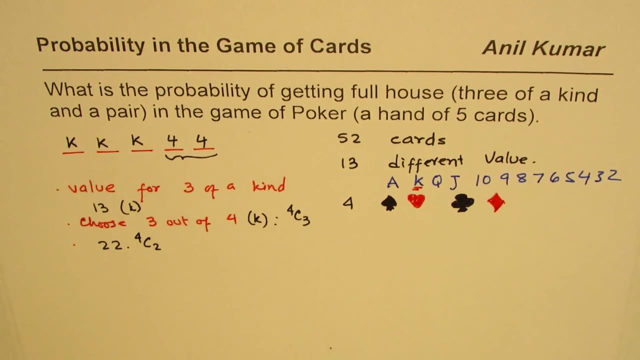 selected 1.. So we are left with 12 different values, right? So that means for the next, this option, we have 12.. And once we decide on the value, we have to select 2 out of 4.. So 12, 4, C, 2. That becomes the combination correct. 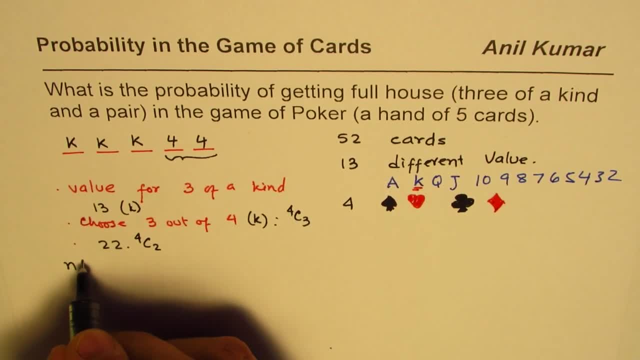 So from the multiplication rules we can say that the probability of our event, let's say event is A favorable chances, are 13,. the value of the first 3 of a kind selecting 3 out of those 4. And then 12 for the pair we have to select. 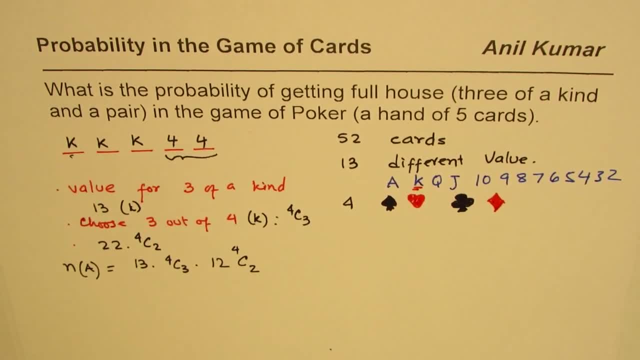 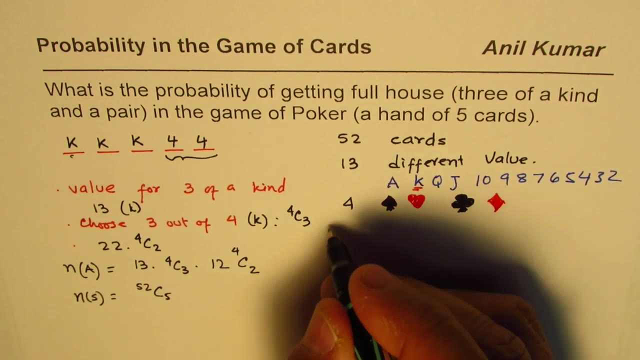 2 out of 4.. So that becomes the favorable chances, right. And total number of outcomes are. we are selecting 5 cards out of 52, right? So that gives us total number of outcomes And now we can easily find the probability. So the probability for this event is the.